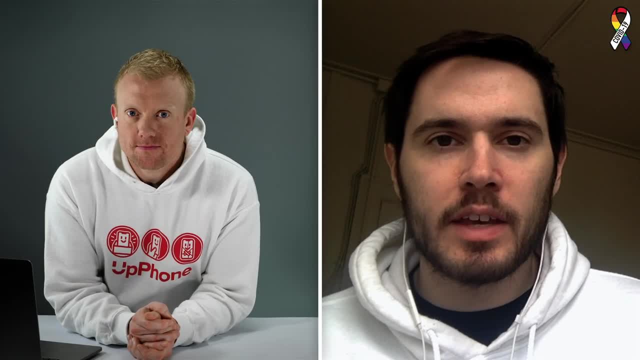 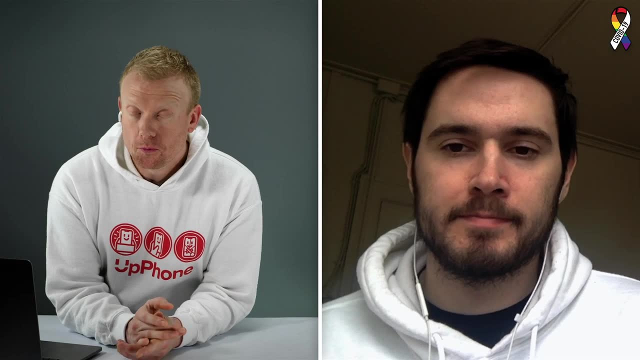 Hey everybody, David and David here from payetteforwardcom and upphonecom, and in this video we're going to explain which cell phones get the best reception. This is a pretty common question and the answer might surprise you, because it really doesn't have a lot to do with the phone itself. 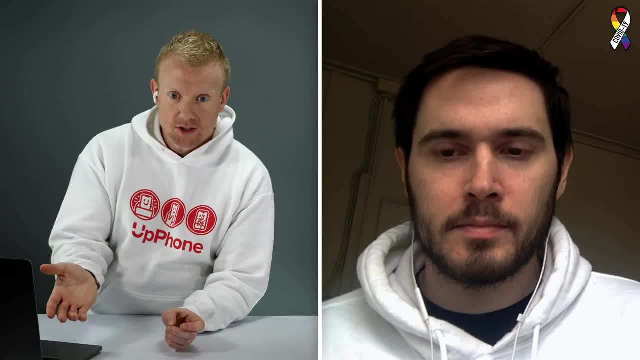 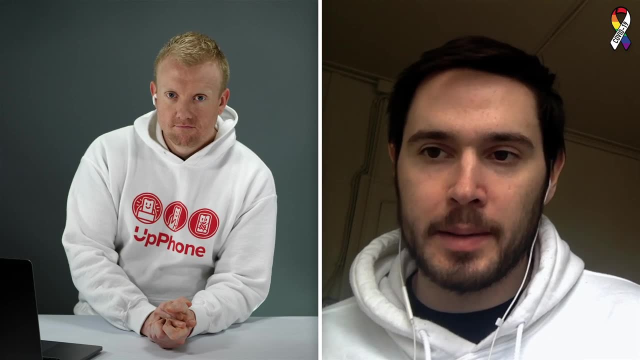 The first big factor is reception right And cell phone coverage Yeah. so it doesn't matter which phone you have. if your carrier doesn't have good service in your area, you're not going to get good reception. So make sure to check out up phones coverage maps just to make sure your carrier does have. 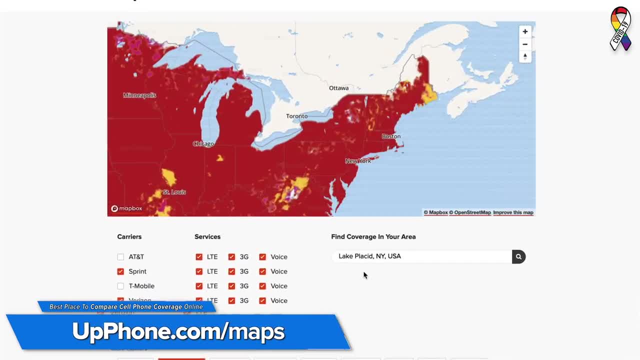 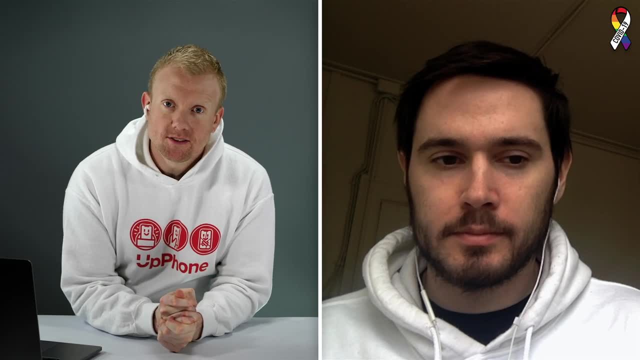 service in your area, because you could have the best phone in terms of reception to talk about in a minute. But if you have no service doesn't matter. The second point we want to make is that pretty much every cell phone out there has very similar. 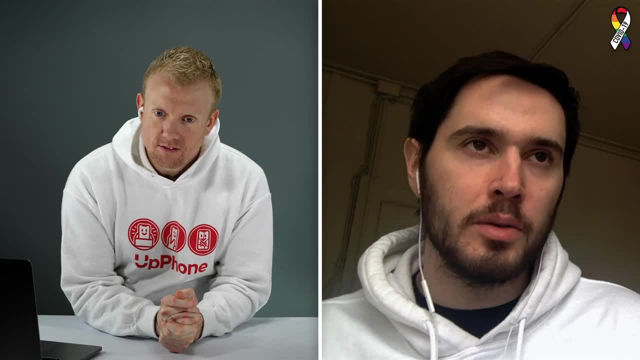 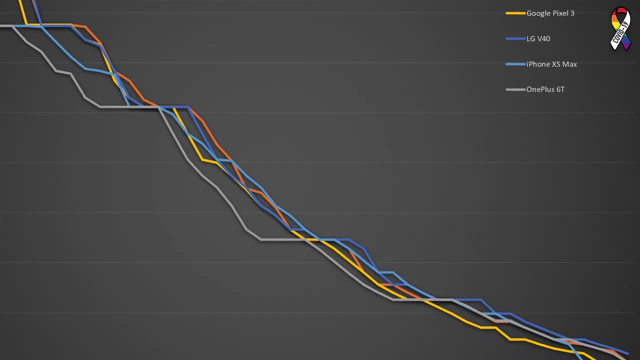 service. right, David? Yeah, all the cell phones. I mean, if you compare the top phones, there's not gonna be a big difference in terms of reception or hardware. PC Magazine did do a study which found the LG V40 did have the best reception. 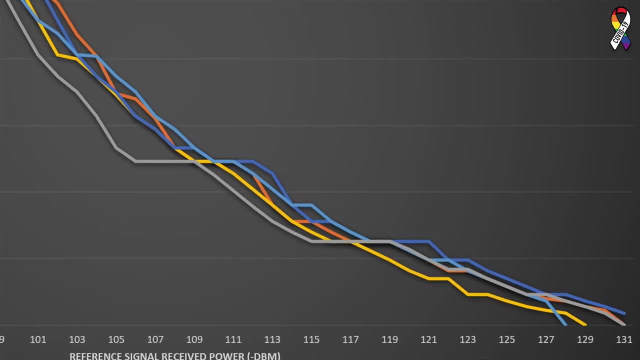 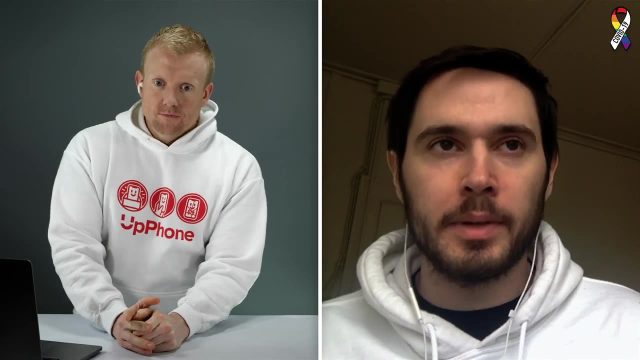 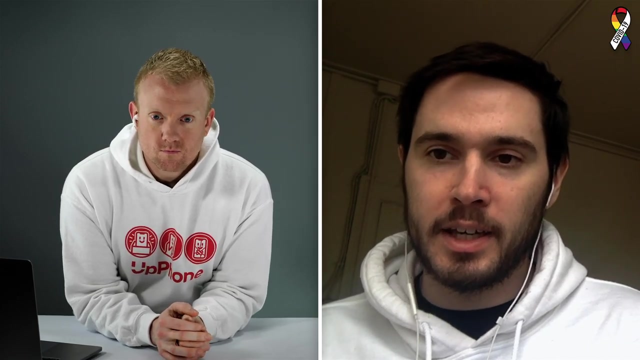 But not significantly. It's not like if you go buy an iPhone 11 Pro Max you're going to get significantly worse reception than the LG V40. So really don't get too concerned about comparing which phones antenna is the best. Think more about your wireless carrier and the phone that you actually like and making. 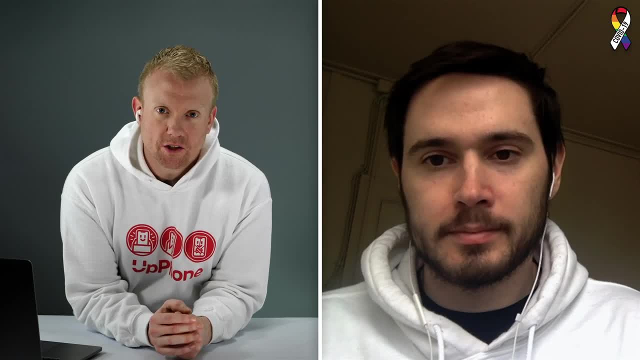 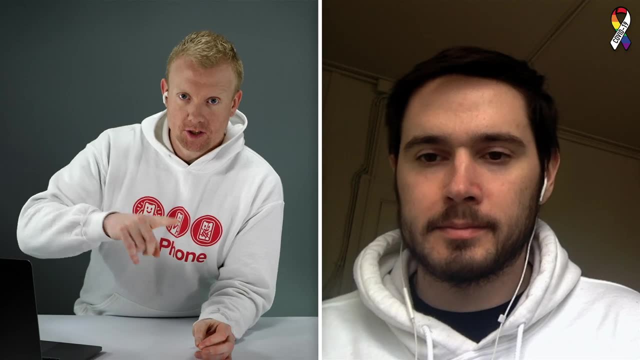 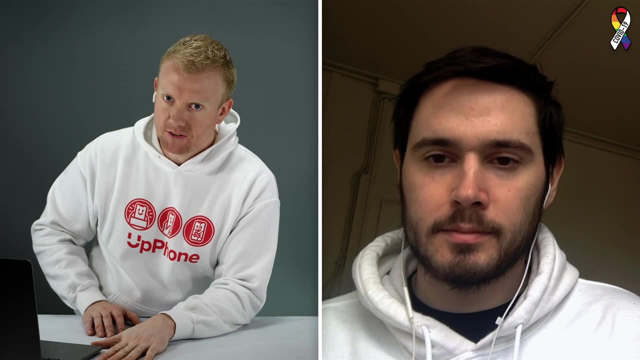 sure that your carrier has good coverage in your area. I think that's really good advice, especially thinking about the phone that you actually want, because inside of the phones, a lot of these companies are using the same chipsets as any companies that are making just antennas for cell phones. Qualcomm is one, Intel is 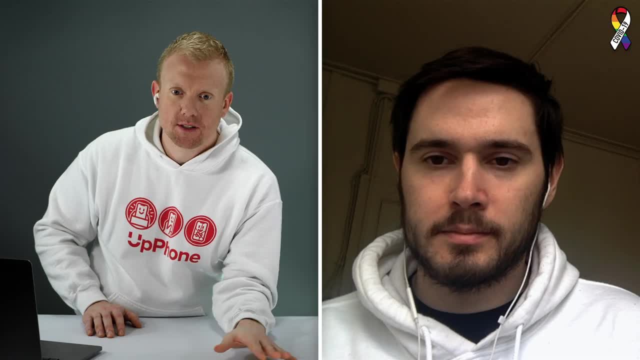 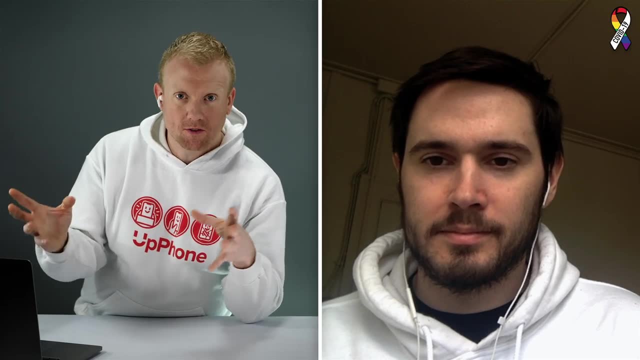 another 2018,. Apple was using the Intel chips, Samsung, LG- they were using the Qualcomm chips. The Qualcomm chips were slightly better than the Intel chips, So it's really more of a question of: is Qualcomm better than Intel? And then the phone has a little bit to do with it. 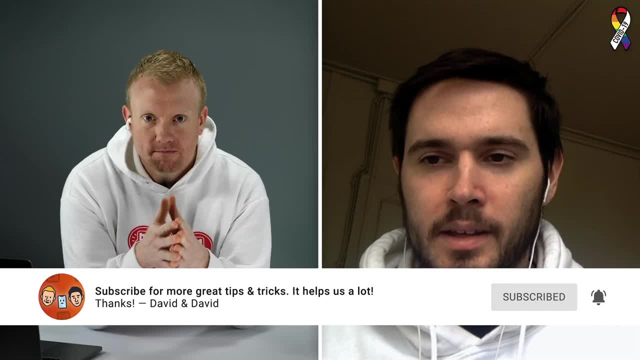 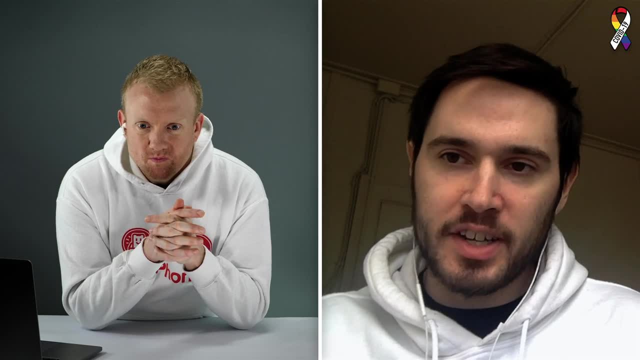 Mostly the antenna, but even though the antennas are pretty much the same, as David said, Yeah, I think if you're a regular user you're not going to notice a difference between the best antenna and average antenna. it's still going to sound pretty similar.